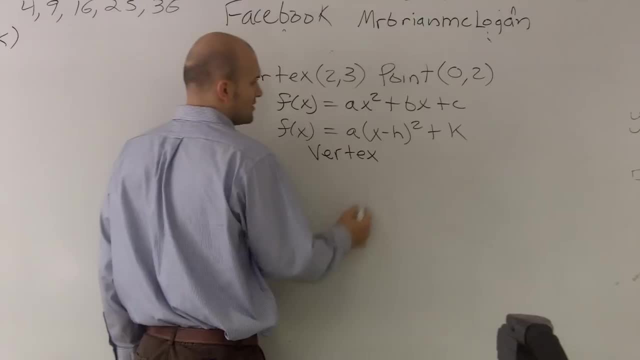 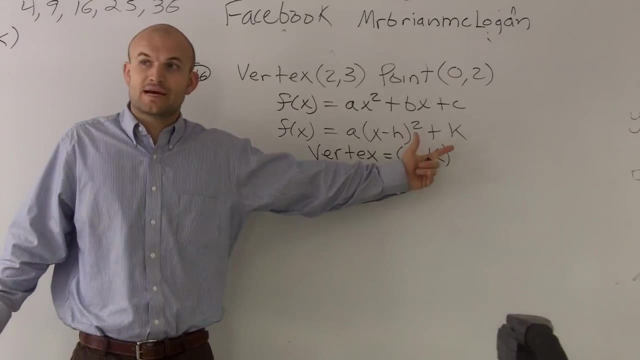 in your guys' notes we have, the vertex is equal to h comma k. So it tells you right there vertex is h comma k. Now there is a formula we can find the vertex for this, but we haven't gotten that yet. So if I 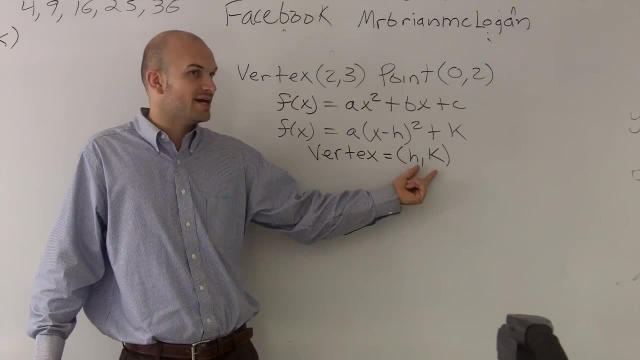 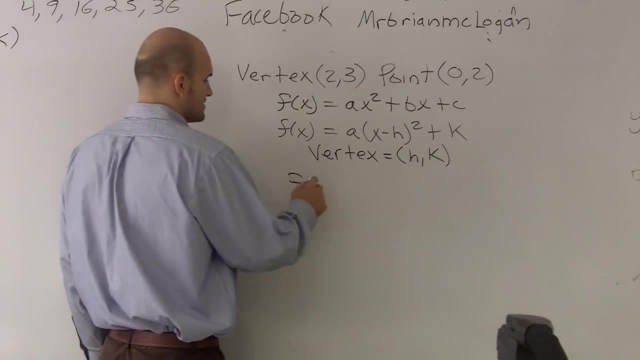 just want to find what is the formula. and they tell me the vertex is hk, and then they tell you what the vertex is. well, it's very easy, Let's just plug that in. So I have f of x equals my vertex, 2 is my h. so 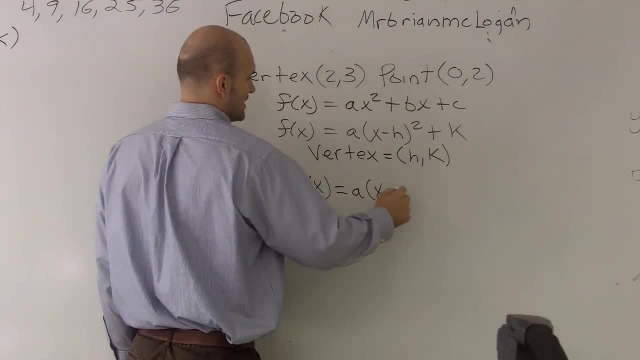 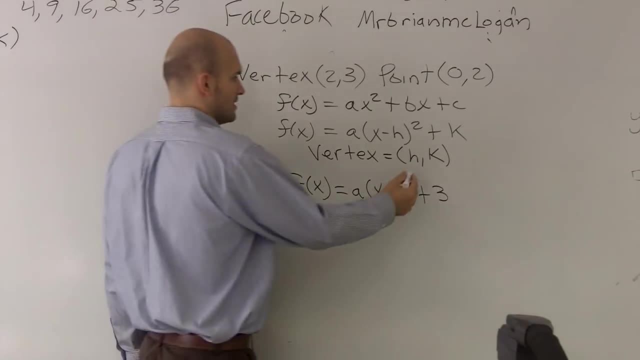 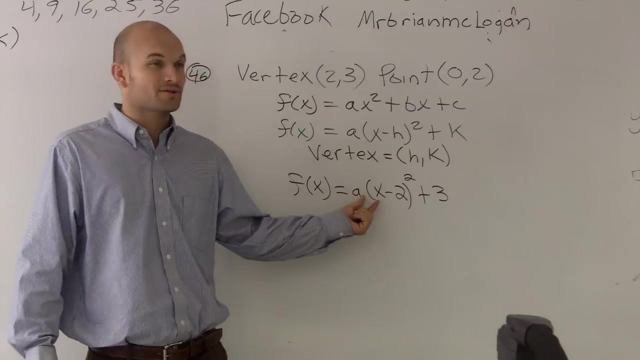 2 goes in for h, so it's ax minus 2 plus 3 is my k And that's a square. obviously All right. Now this isn't fully completed because one thing: I don't know what a is. I have two variables now. 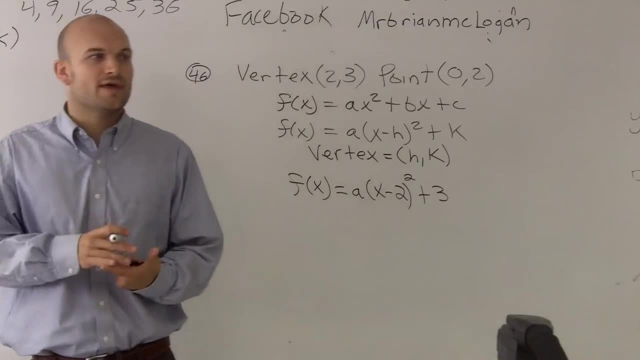 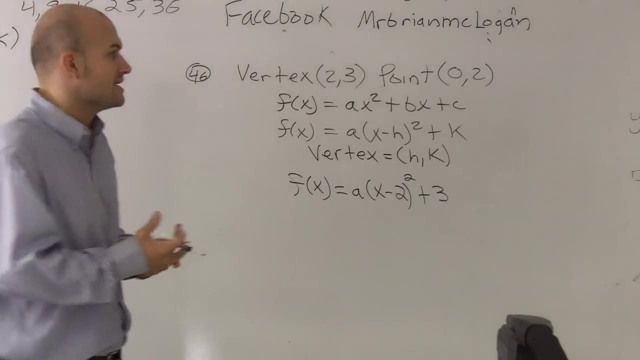 I have an a and an x, So I need to find the value of a. So to do that, one thing they tell us is this: graph goes through this point And remember, a graph is a set of, you know, is a set of points. 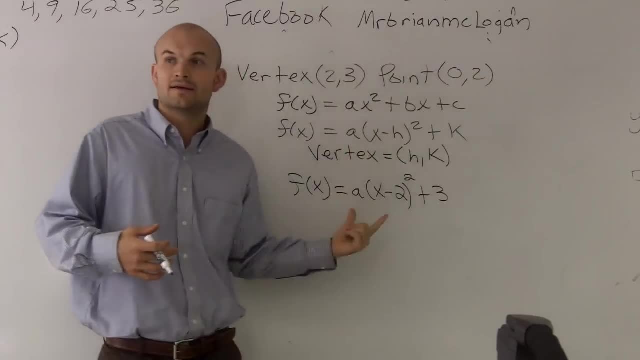 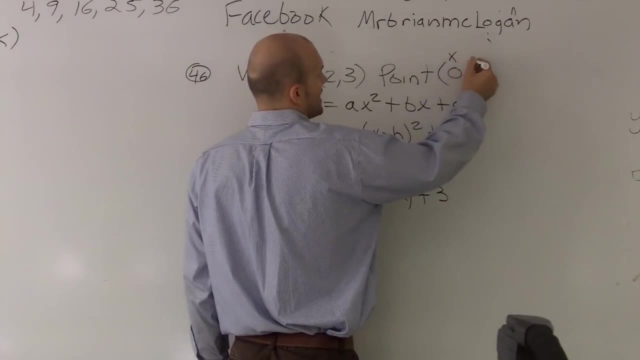 Therefore, I know this point is on my graph, So if I plug this point in, it's going to make this equation equal and it'll tell me what the value of a is. So one thing you can think about now that we're talking about functions is: remember functions are input. You have an input value. 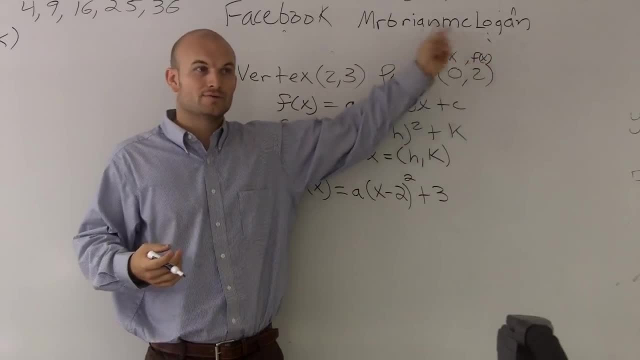 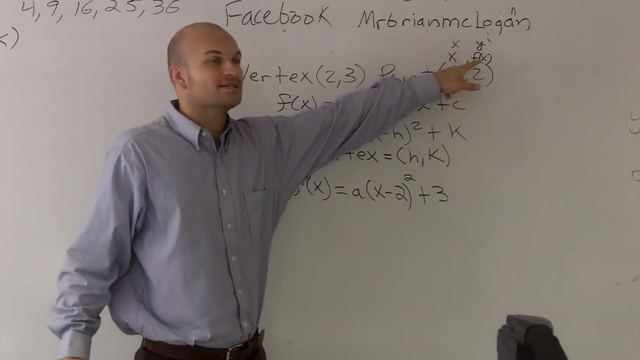 and an output value, right Input and output domain and your range. It's the same thing as x and y. So my output value, my y variable, is the same thing as my f of x. So I'm going to plug in 2,. 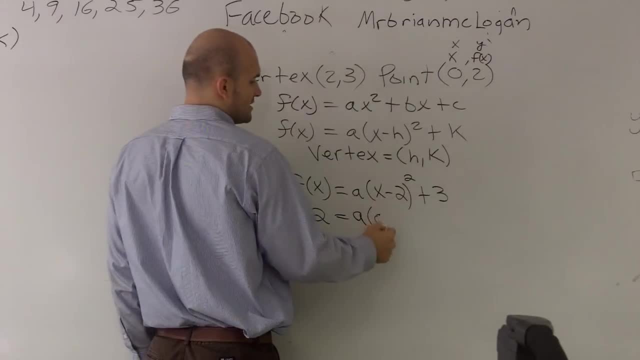 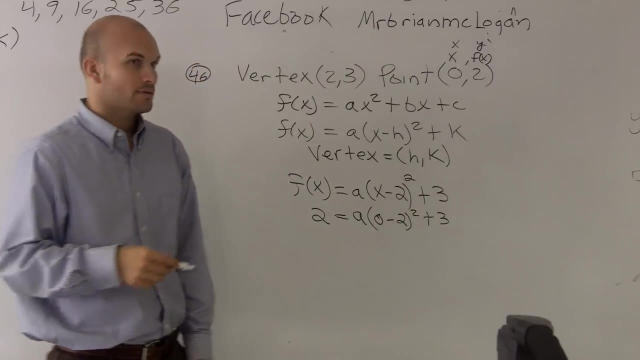 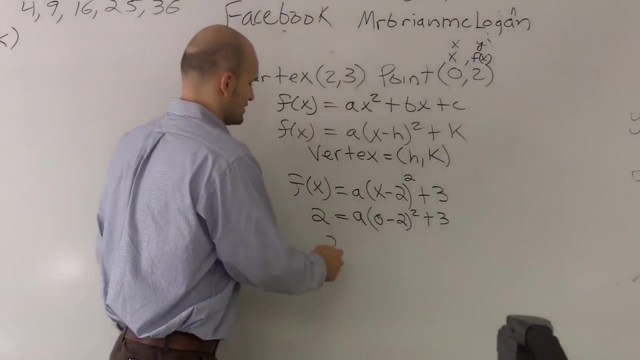 which is equal to a. I don't know the value 0, they tell us is 0. I'm sorry, x is 0, minus 2 squared plus 3.. So then, 0 minus 2 is going to give you negative 2.. Negative 2 is 4.. So I get 2. 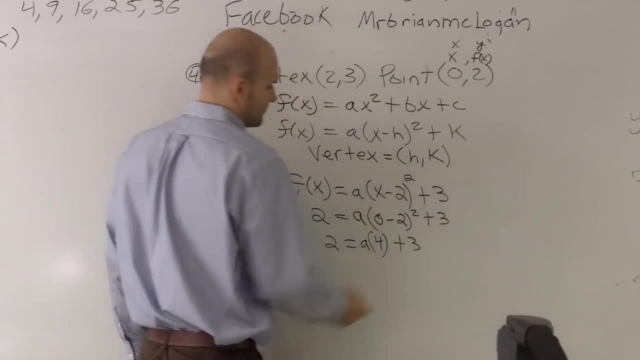 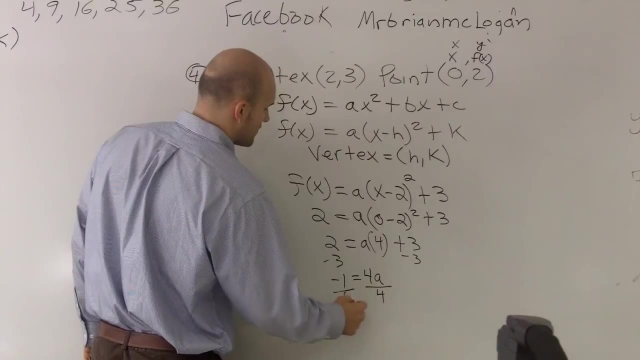 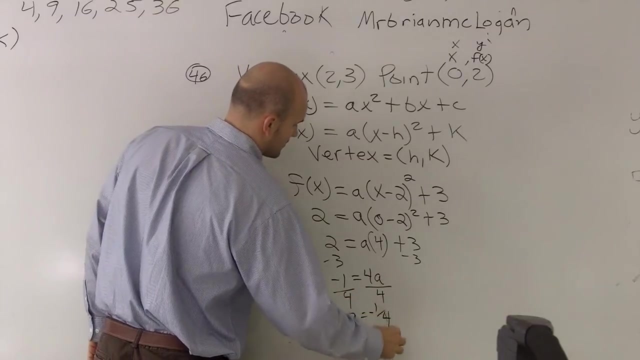 equals a times 4 plus 3.. Subtract the: 3. Negative 1 equals 4a. Divide by 4. a equals a negative 1 4th. That's right there. Any questions Make sense? Not done yet, But at this. 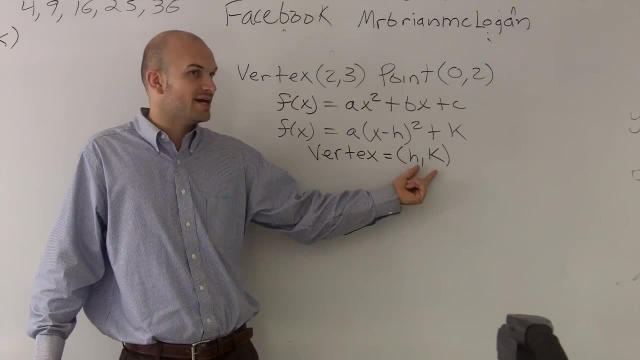 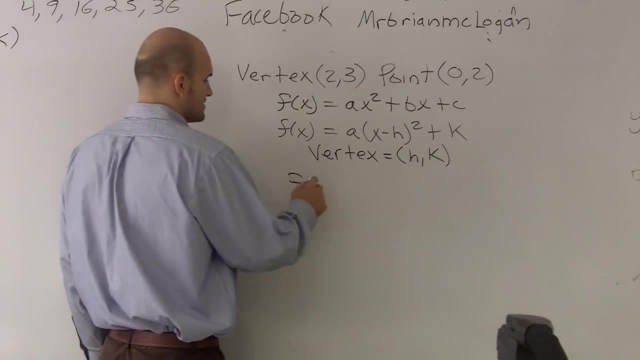 just want to find what is the formula. and they tell me the vertex is hk, and then they tell you what the vertex is. well, it's very easy, Let's just plug that in. So I have f of x equals my vertex, 2 is my h. so 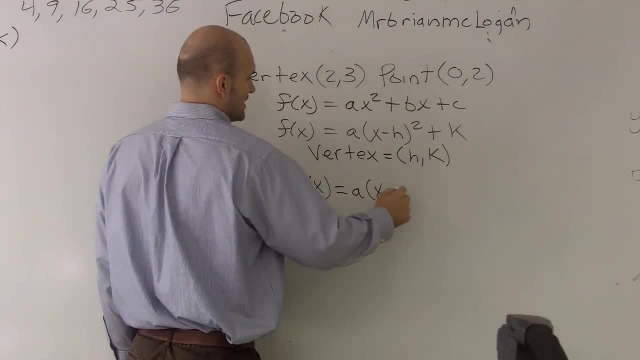 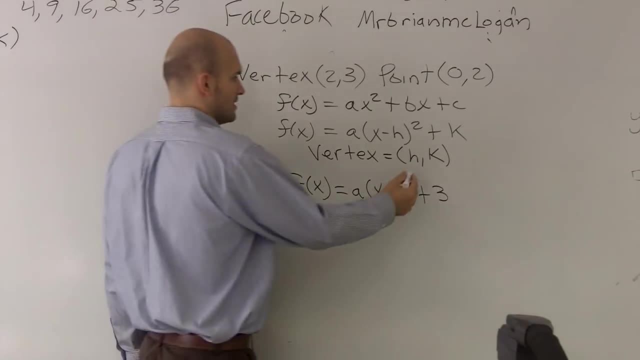 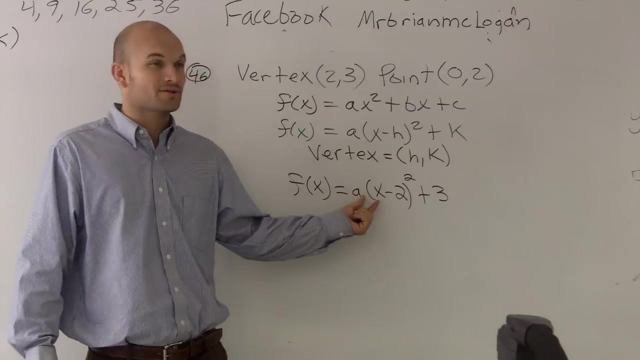 2 goes in for h, so it's ax minus 2 plus 3 is my k And that's a square. obviously All right. Now this isn't fully completed because one thing: I don't know what a is. I have two variables now. 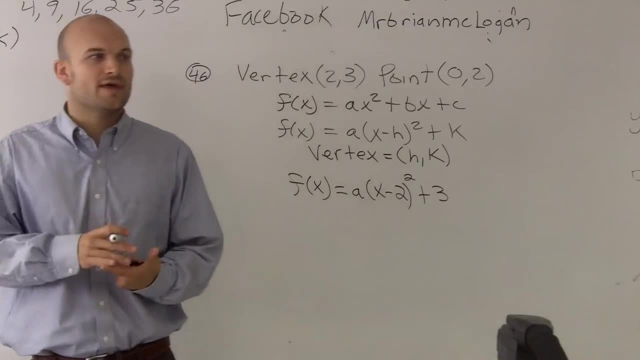 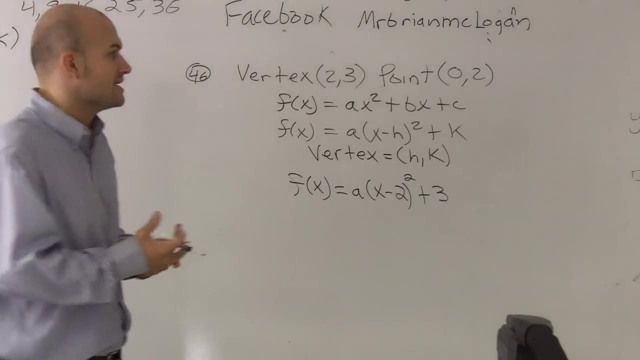 I have an a and an x, So I need to find the value of a. So to do that, one thing they tell us is this: graph goes through this point And remember, a graph is a set of, you know, is a set of points. 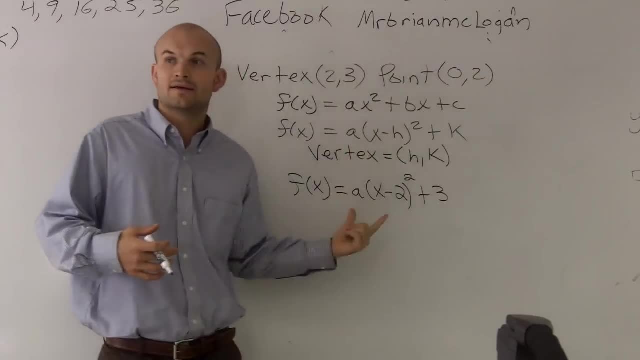 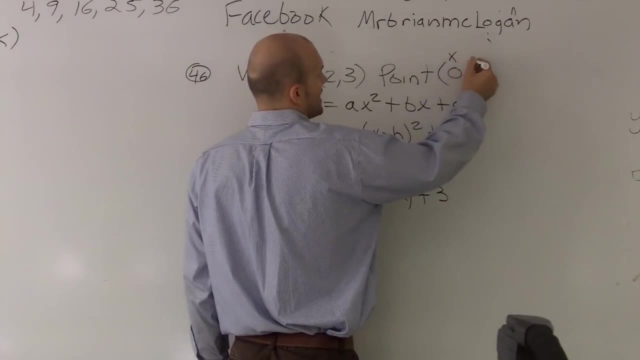 Therefore, I know this point is on my graph, So if I plug this point in, it's going to make this equation equal and it'll tell me what the value of a is. So one thing you can think about now that we're talking about functions is: remember functions are input. You have an input value. 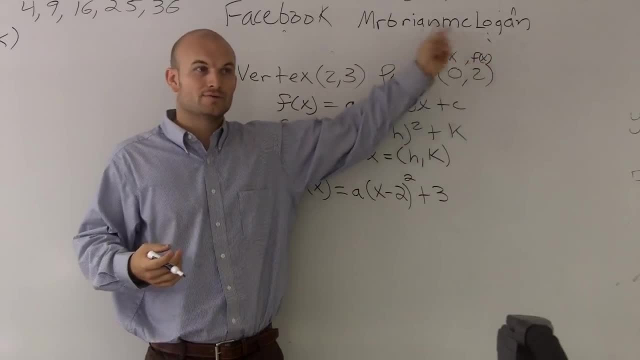 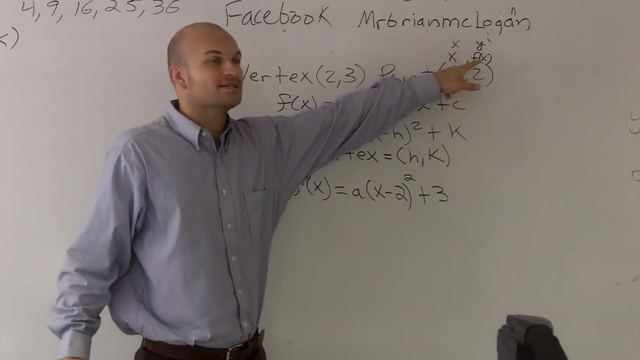 and an output value, right Input and output domain and your range. It's the same thing as x and y. So my output value, my y variable, is the same thing as my f of x. So I'm going to plug in 2,. 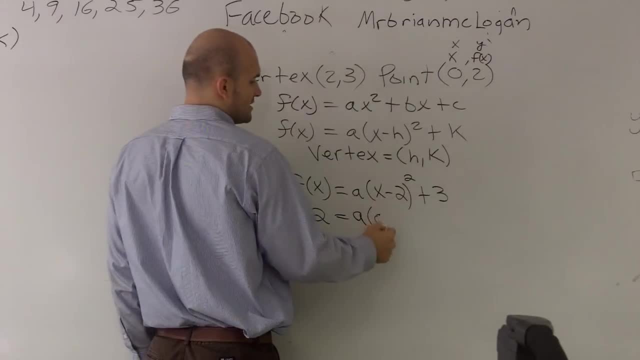 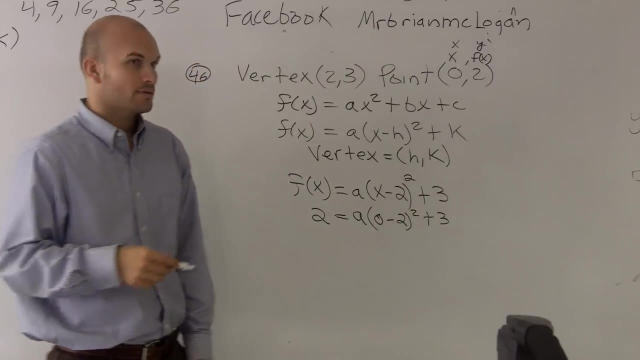 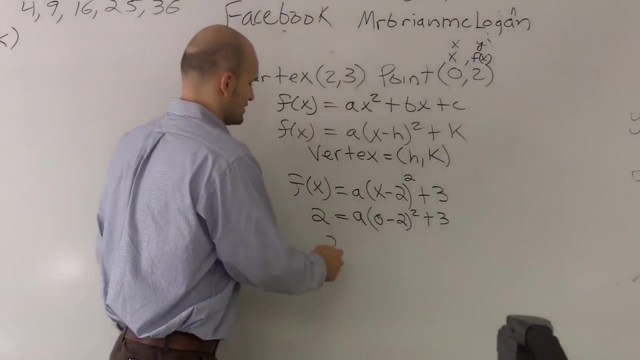 which is equal to a. I don't know the value 0, they tell us is 0. I'm sorry, x is 0, minus 2 squared plus 3.. So then, 0 minus 2 is going to give you negative 2.. Negative 2 is 4.. So I get 2. 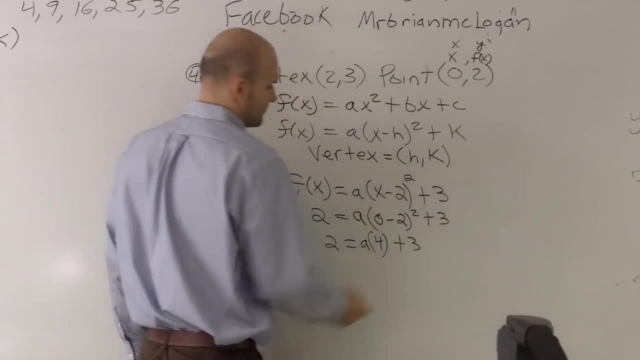 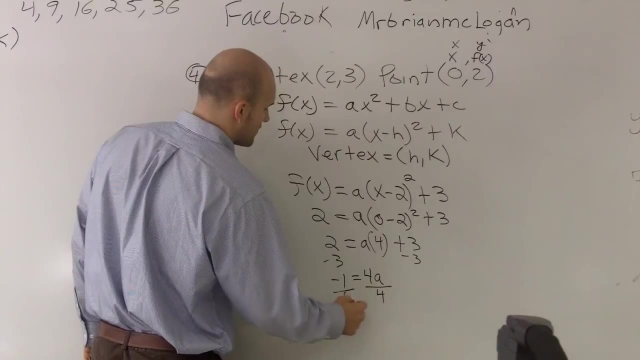 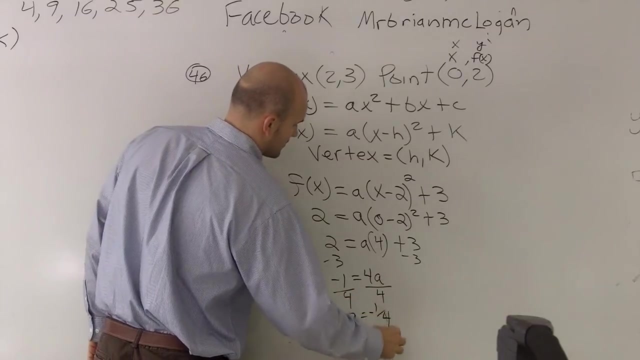 equals a times 4 plus 3.. Subtract the: 3. Negative 1 equals 4a. Divide by 4. a equals a negative 1 4th. That's right there. Any questions Make sense? Not done yet, But at this. 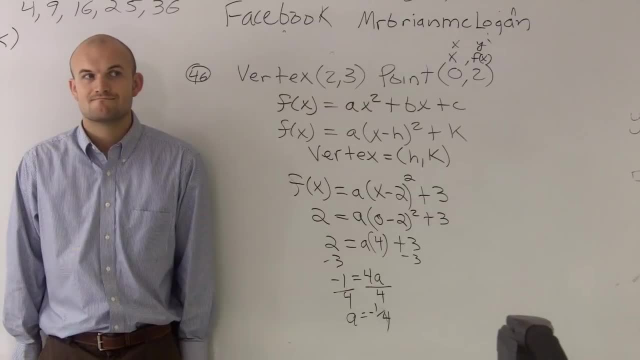 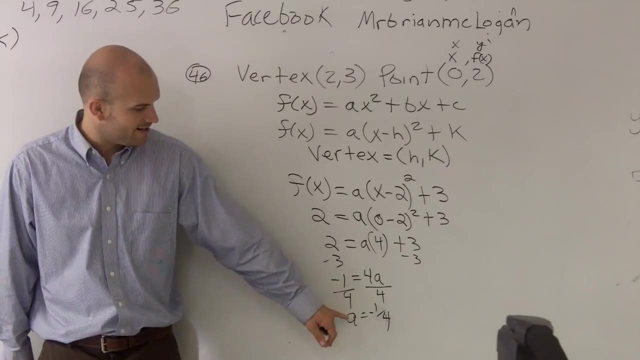 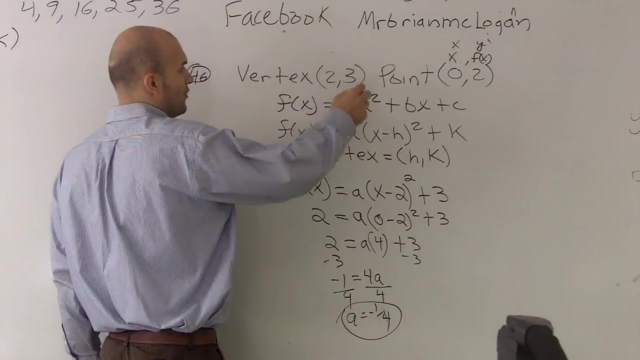 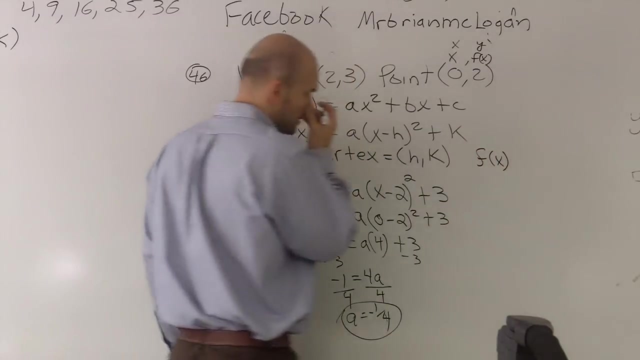 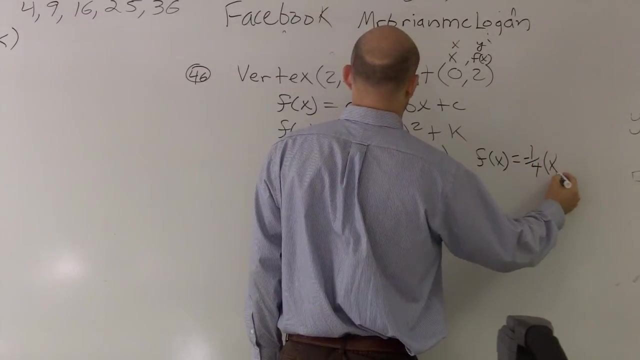 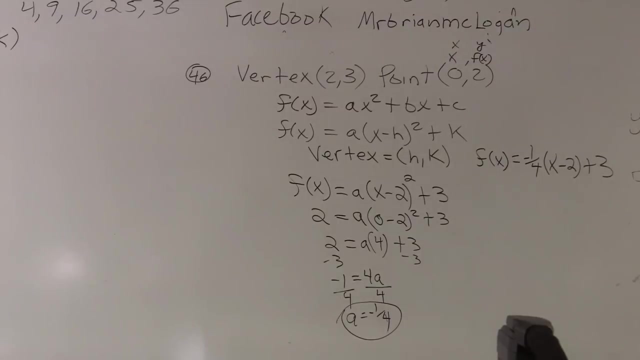 point. we got it, Yes, Maybe All right. And then from here I just plug in my a back to my equation. So now I know what a is, I know what my h is And I know what my k is. So f of x. f of x equals a negative 1, 4th x minus 2 plus 3. And Minus 2 squared. 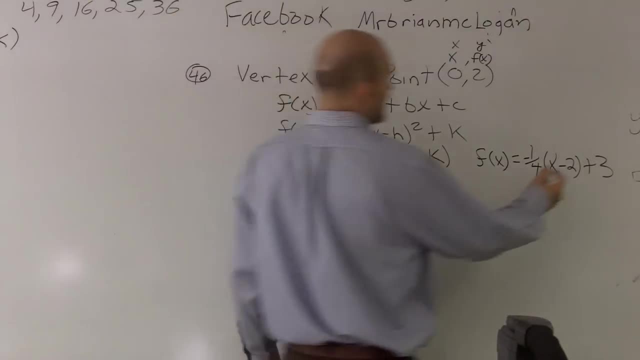 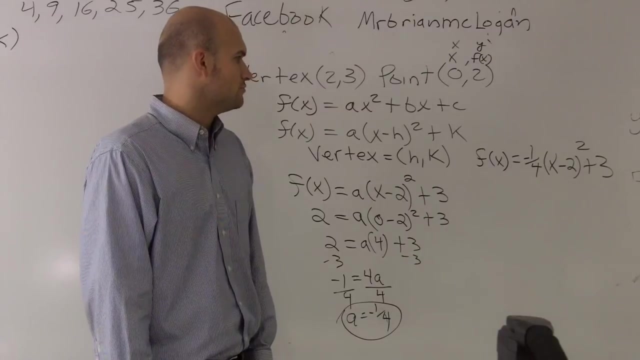 That's all there, I'm sorry. Minus 2 squared. Yeah, minus 2 squared. And then: Yeah, Yes, There you go, And then 2.. And if you wanted to do it at the quadratic form, if the question asks, we'll put it right in as a. 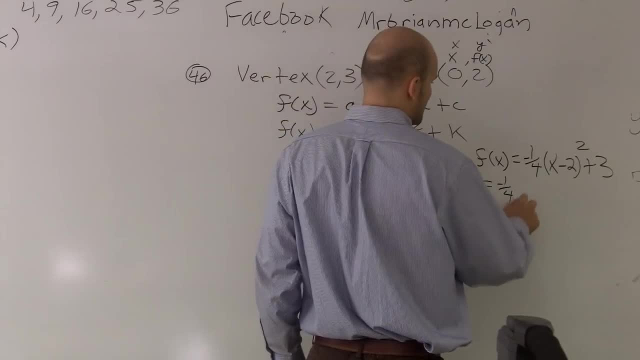 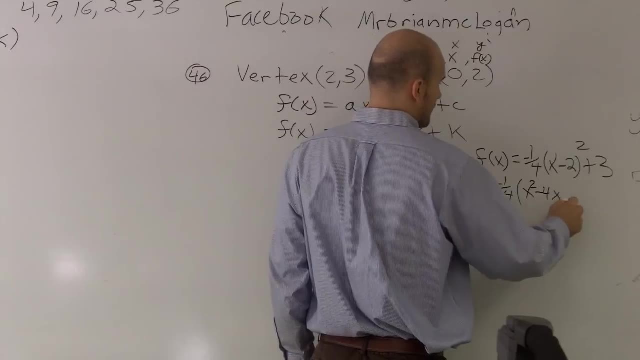 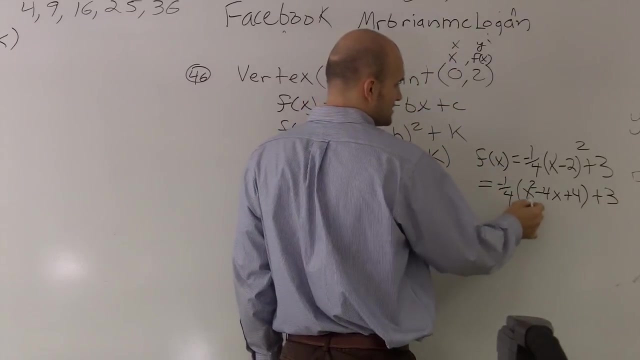 quadratic, Then you'd have to do negative 1 4th Factor, that x minus 2 times x minus 2.. x squared minus 4x plus 4.. Right Plus 3.. Then you have to distribute this. Is it going to ask us to do it in? 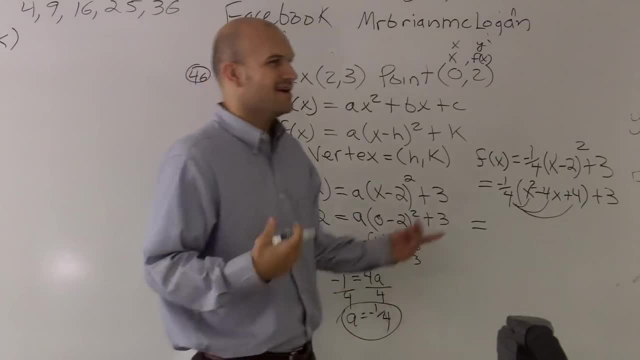 quadratic form. I'm just saying maybe It might ask you to do it in quadratic, But usually it's. there's really no point. But I just want to kind of see how you guys can see where you're going from here to a. 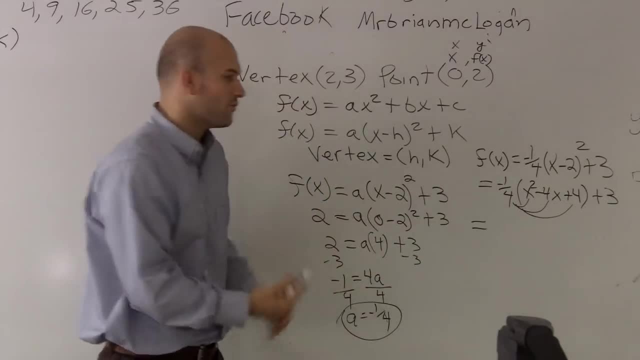 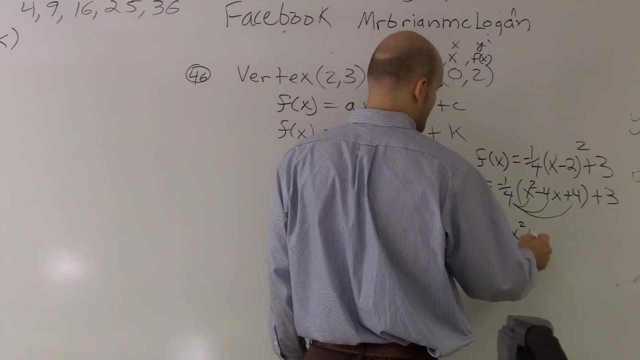 standard form to a quadratic form, How they're all related. It's just different forms. So this would be a negative 1 4th x squared. These are now going to cancel out Right Plus x minus 1 plus 3.. 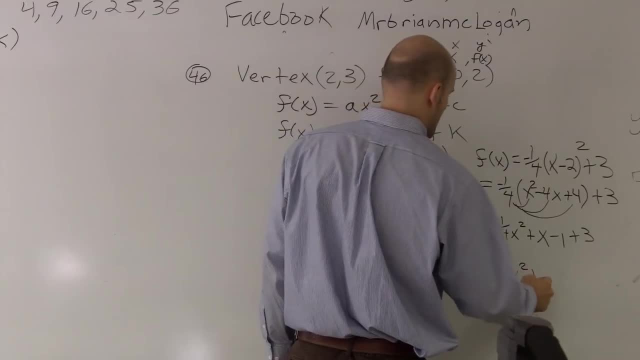 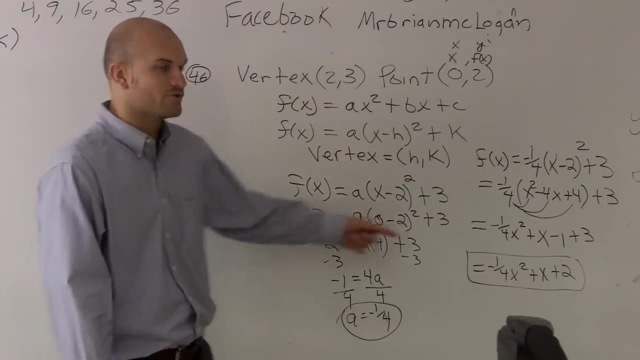 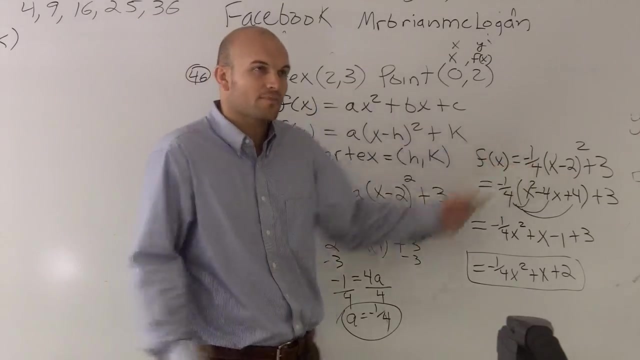 So we're trying to get it in standard form. No, we already put it in standard form. We're trying to put it in If we wanted. if I asked you if it was in quadratic form Before that, Yeah. All I was asking to do, though, was yes, it was. I just asked you to put it in standard form. 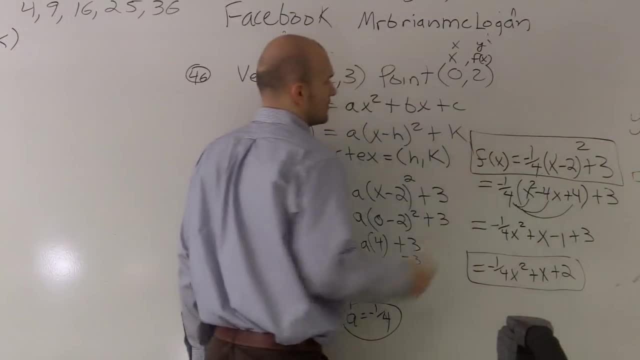 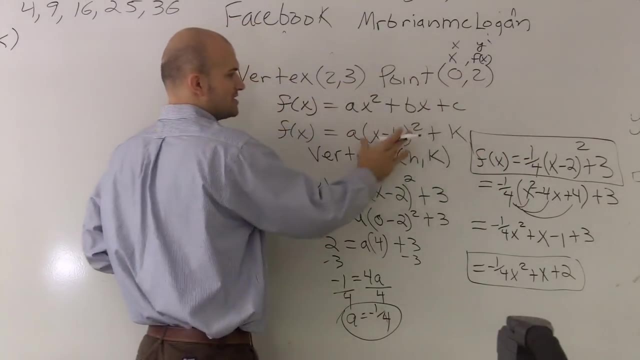 Which would have been perfectly acceptable. Can you do it from standard form? What do you mean? Did you just do it from? Yeah, all I did was I take my vertex and my point, I plugged them into my standard, I plugged them into the standard form equation And I followed the equation of my graph in standard form. 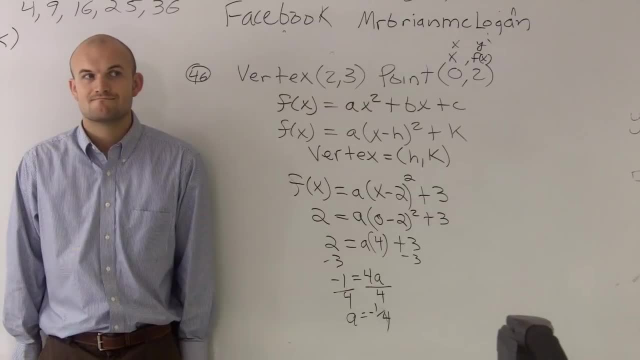 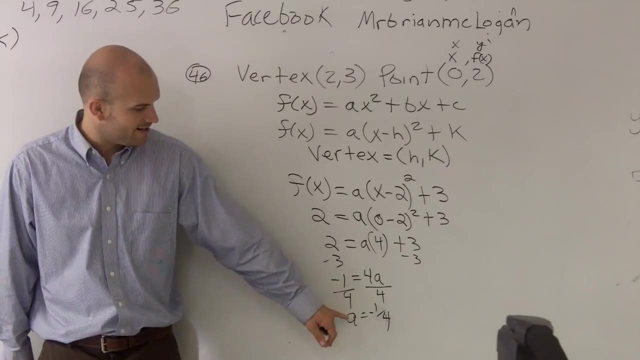 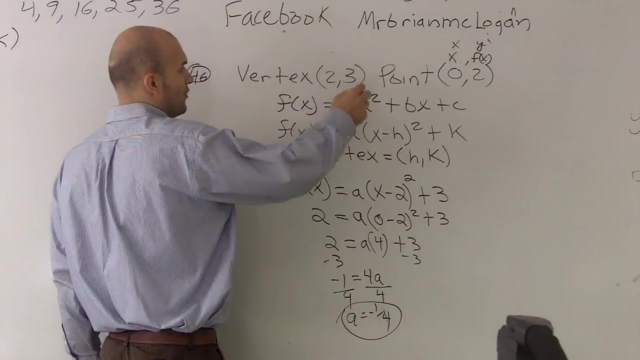 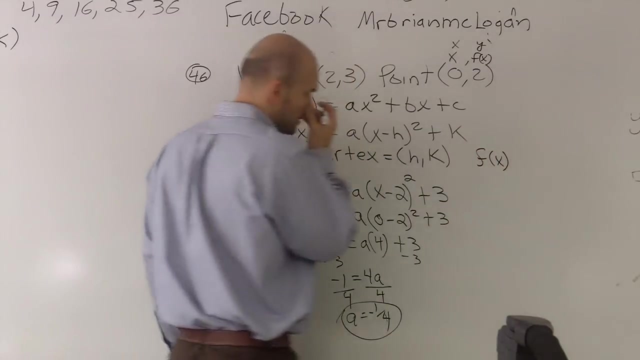 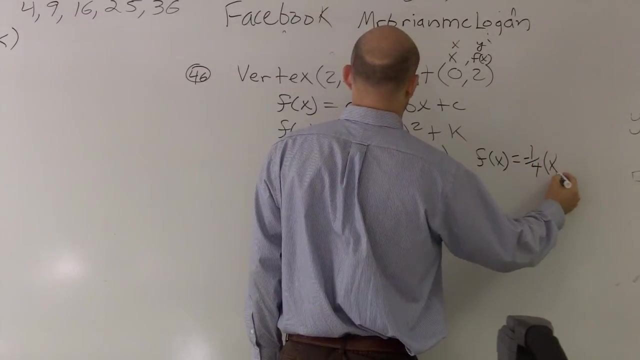 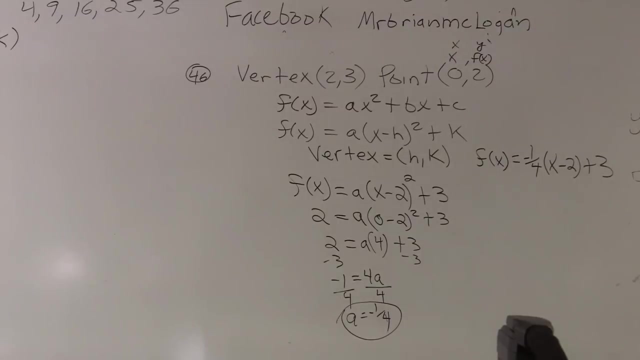 point. we got it, Yes, Maybe All right. And then from here I just plug in my a back to my equation. So now I know what a is, I know what my h is And I know what my k is. So f of x. f of x equals a negative 1, 4th x minus 2 plus 3. And Minus 2 squared. 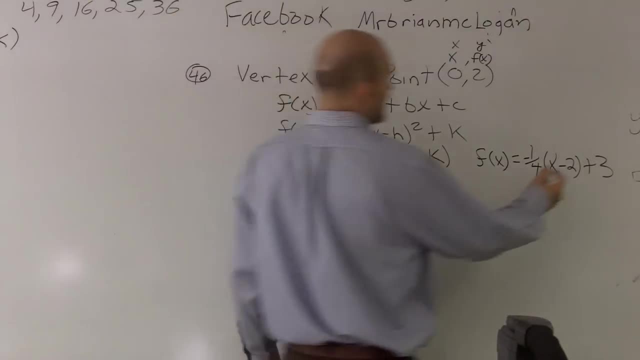 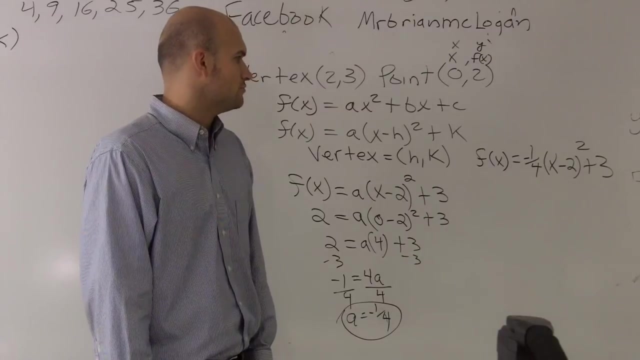 That's all there, I'm sorry. Minus 2 squared. Yeah, minus 2 squared. And then: Yeah, Yes, There you go, And then 2.. And if you wanted to do it at the quadratic form, if the question asks, we'll put it right in as a. 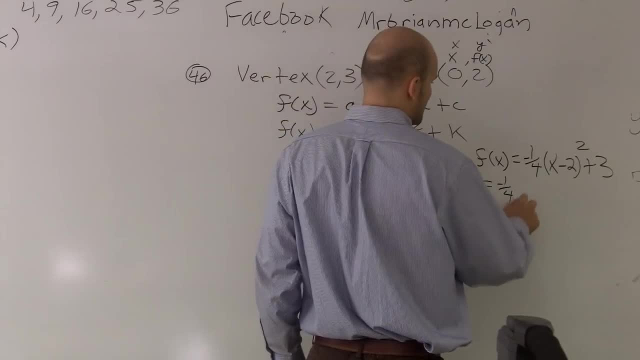 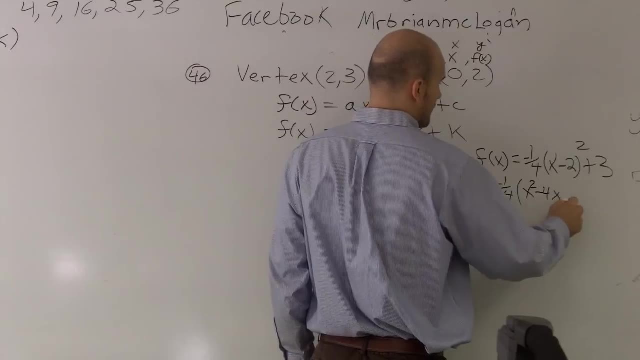 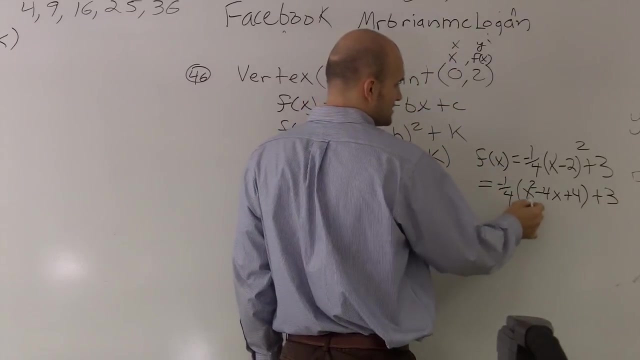 quadratic, Then you'd have to do negative 1 4th Factor, that x minus 2 times x minus 2.. x squared minus 4x plus 4.. Right Plus 3.. Then you have to distribute this. Is it going to ask us to do it in? 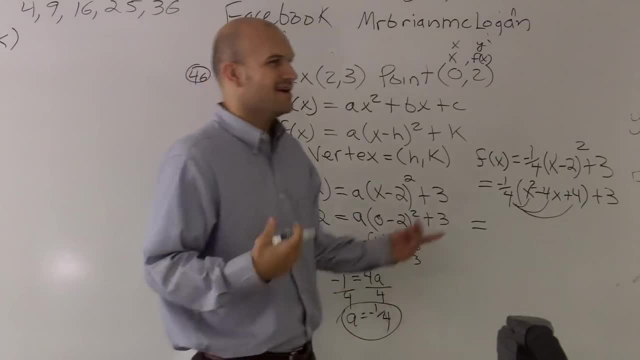 quadratic form. I'm just saying maybe It might ask you to do it in quadratic, But usually it's. there's really no point. But I just want to kind of see how you guys can see where you're going from here to a. 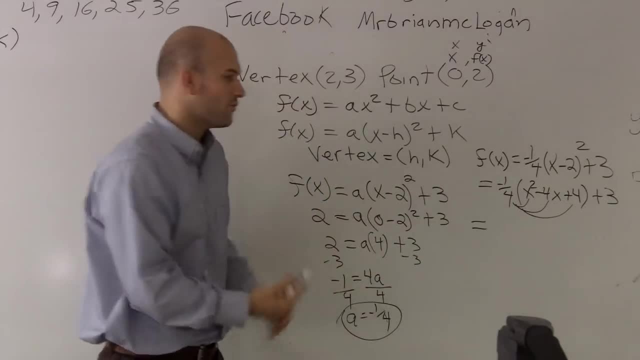 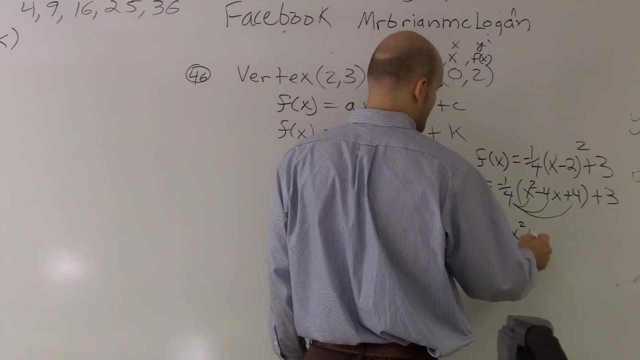 standard form to a quadratic form, How they're all related. It's just different forms. So this would be a negative 1 4th x squared. These are now going to cancel out Right Plus x minus 1 plus 3.. 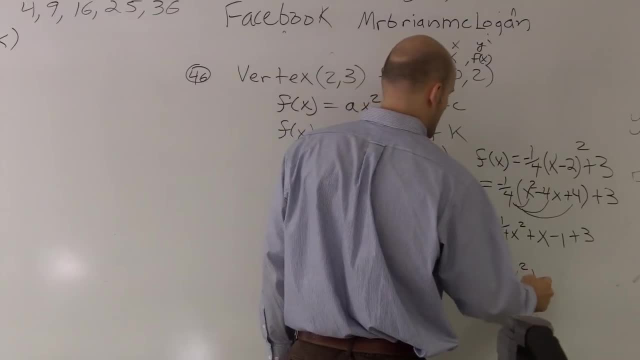 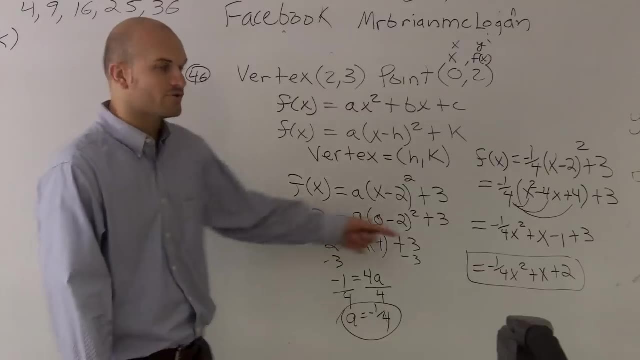 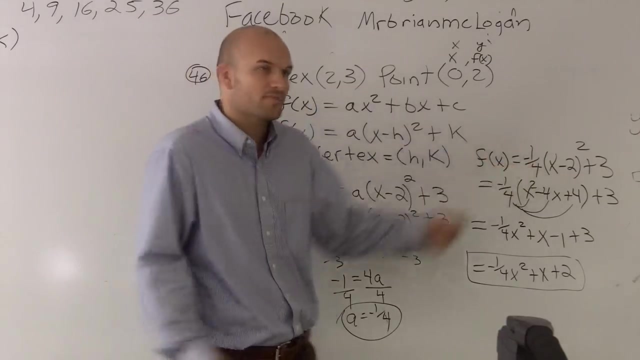 So we're trying to get it in standard form. No, we already put it in standard form. We're trying to put it in If we wanted. if I asked you if it was in quadratic form. No, I mean before that, Yeah. All I was asking to do, though, was: yes, It was, I just asked you to put in standard. 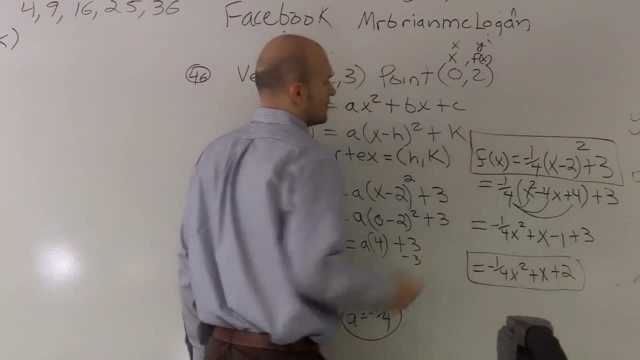 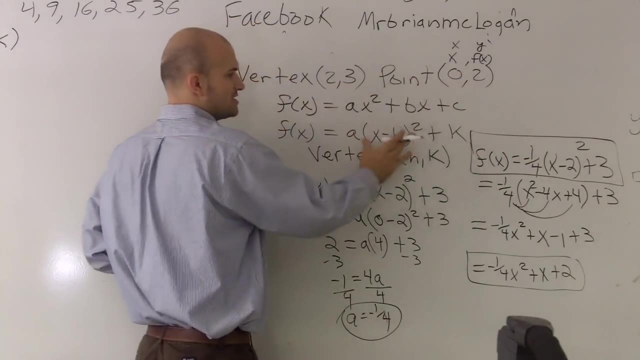 form, which would have been perfectly acceptable. Can you do it from standard form? What do you mean? Could you just do it from standard form? Yeah, All I did was I took my vertex and my point, I plugged them into my standard. I plugged them into the standard form equation. 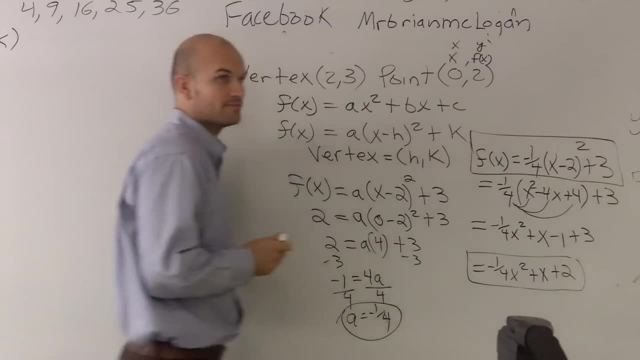 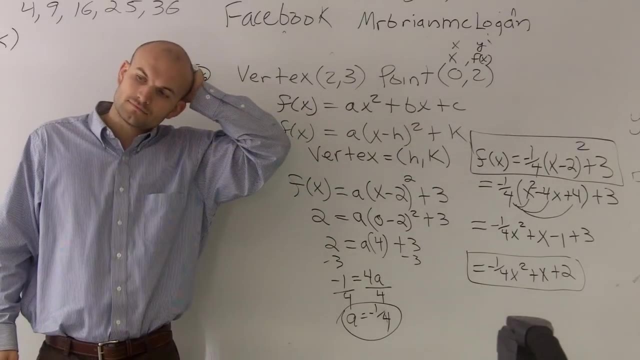 And I found the equation of my graph in standard form. Wait, did you plug your point? Oh, so that's the answer, right there, Yeah, right, Oh, okay. So basically you're just taking the number. I'm sure you remember what you did.